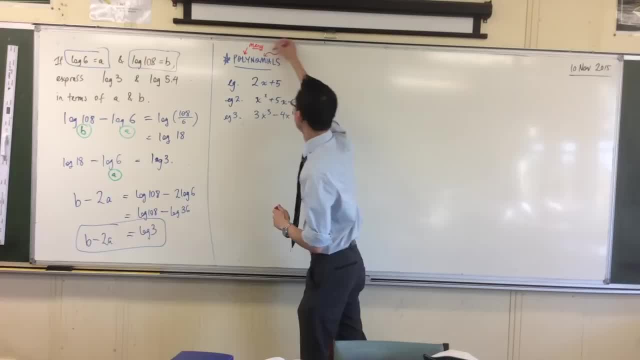 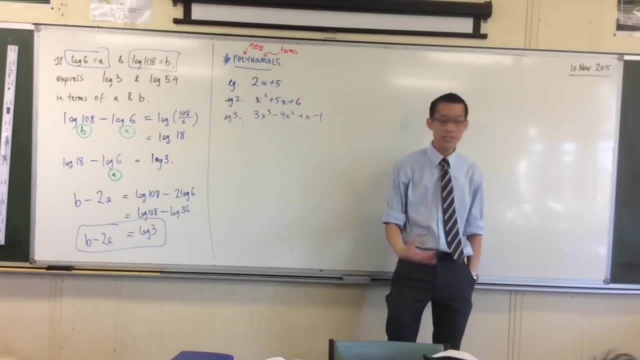 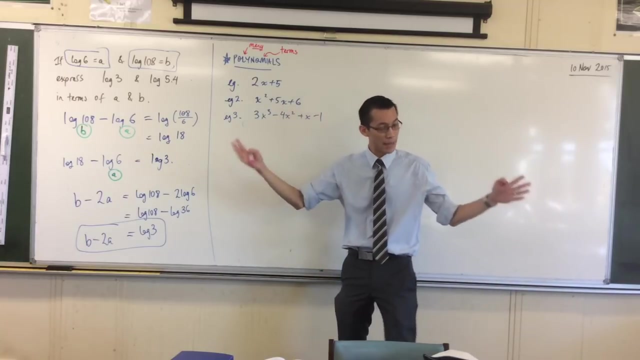 So it means many Nomials. that's a weird phrase In our context. what it means is terms. It's something which has many terms. You can see I've got a whole bunch of terms. I can have as many terms as I like. I don't have to stop at. you know, x cubed, I can make them big or small or whatever I like. okay. 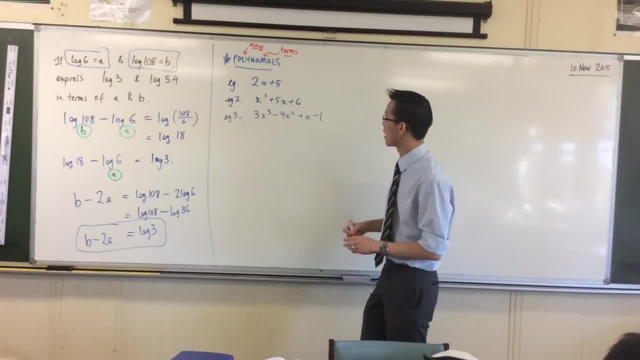 There's a very specific example of polynomials, which is this guy over here. This here is called a binomial because it has two terms in it. right, This is a binomial. By extension, you'd call this a trinomial, and so on. okay. 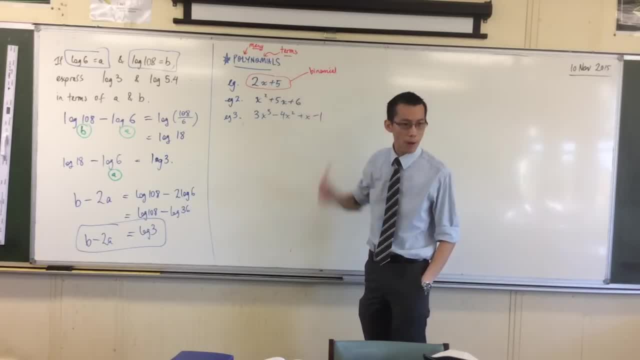 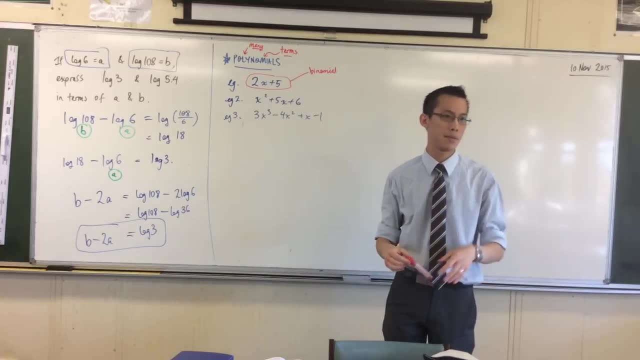 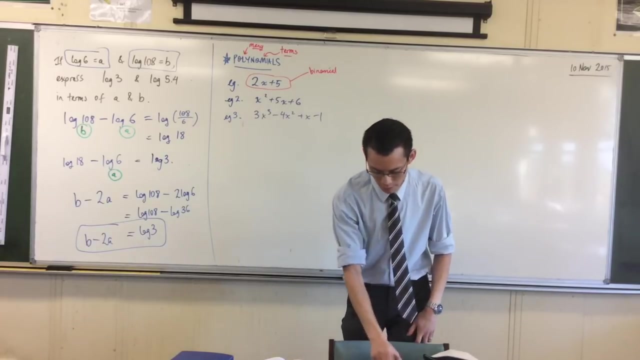 So all that means is I've just got a whole bunch of terms, but the terms are very specific. Can you see? you've always got something and they're raised to powers, and then you've got numbers out the front. okay, So let's introduce some language and we'll use this guy here. No, actually, I'll do one more example. 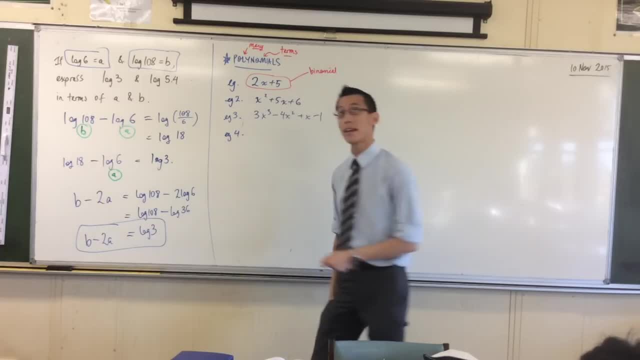 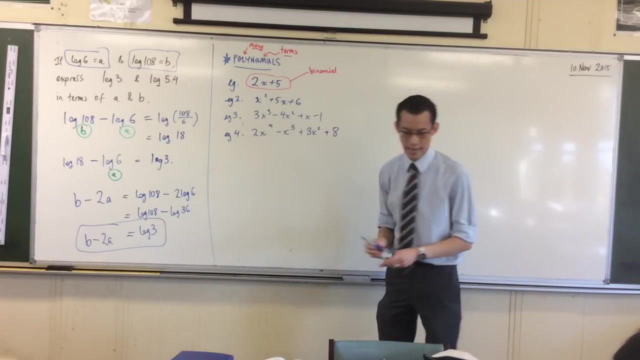 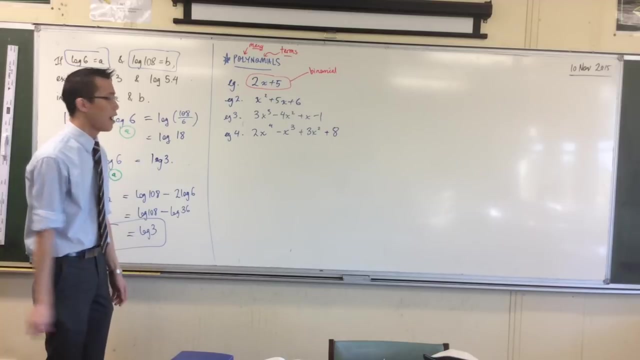 Example four: Let's make it 2x. God bless you. Okay, here we go. So I'm just going to use this as my example and we're going to attach some language to this, okay? Firstly, these are all polynomials. These are all polynomials. 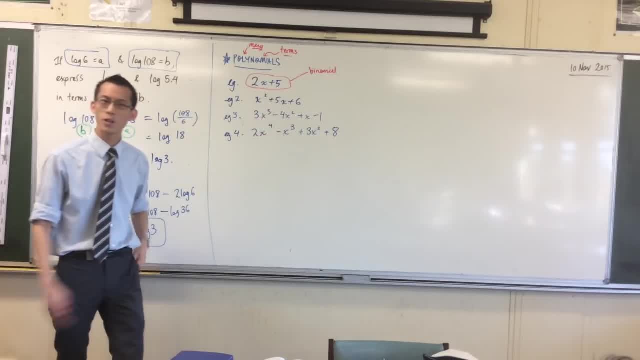 But the reason why I've given you these four as my first examples is because they come up so frequently. they all have special names. When you have things that come up again and again and again, people are like: ooh, that's kind of cool. let's talk about that one. 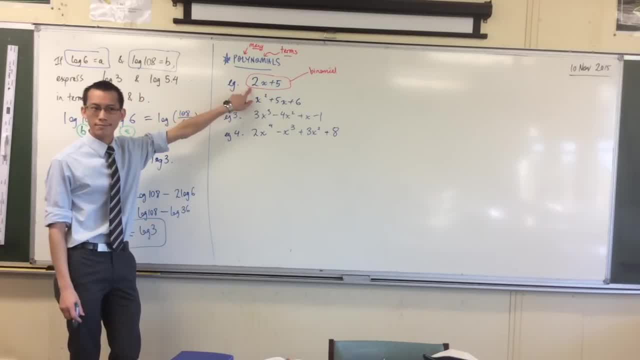 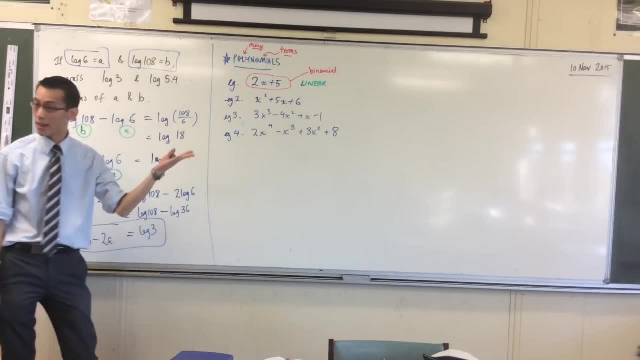 So the first one that we've got, Because if you draw this thing, you'll get a straight line. okay, This is called a linear polynomial. okay, If you draw, y equals 2x plus 5, you just get a straight line, okay. 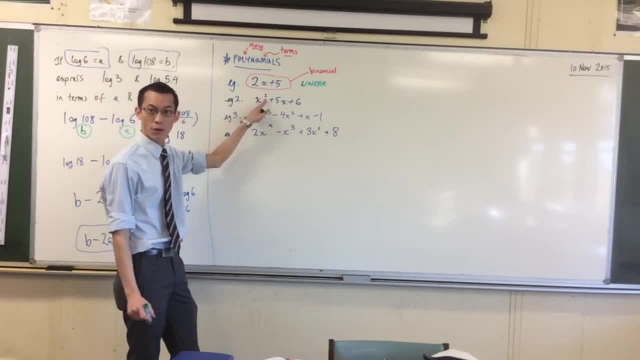 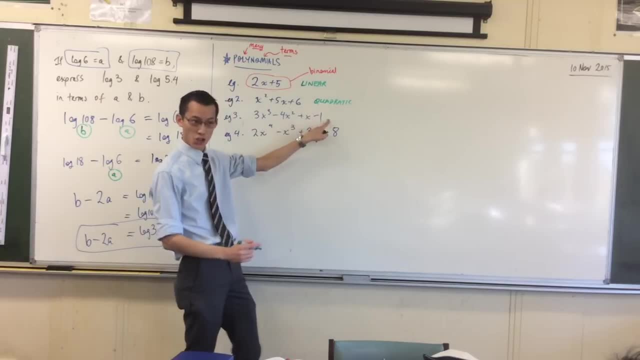 We already know what these guys are called, whether this power up here is a 2. We call these quadratics, right? So this is a quadratic polynomial. A couple of minutes ago you told me this is a cubic polynomial And this last one here, like you can see, these have to do with the number. 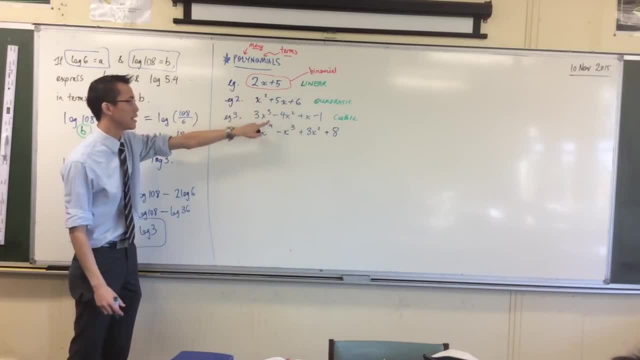 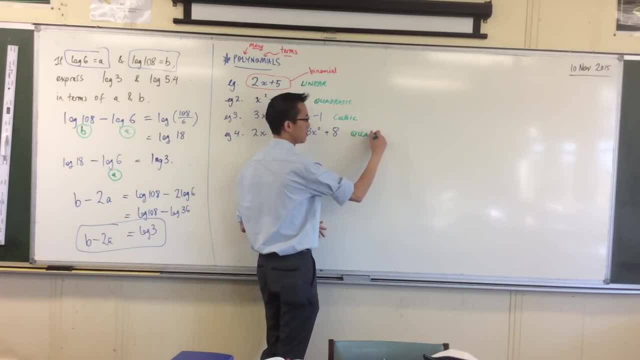 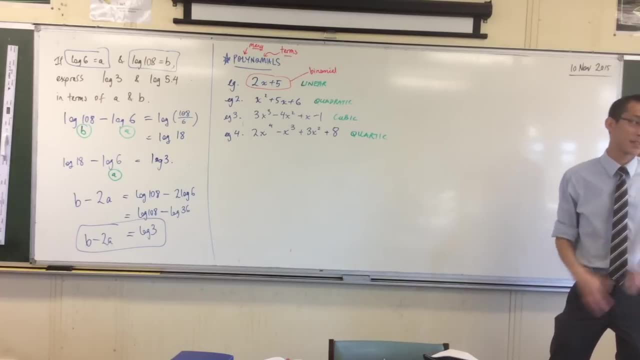 So these guys here are called quartics. okay, If it's a power 5, you get a quintic, And after that you kind of They stop calling them special names because they don't come up very often. okay, At least in the mathematics that we're doing. 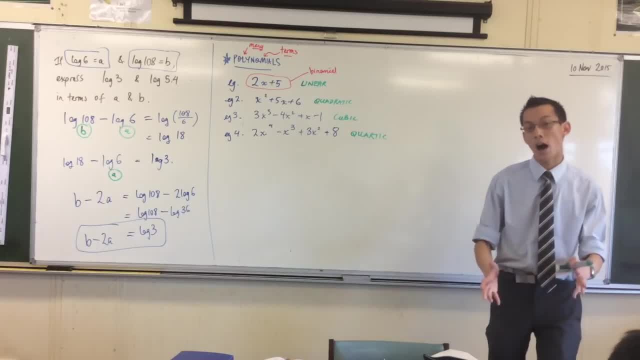 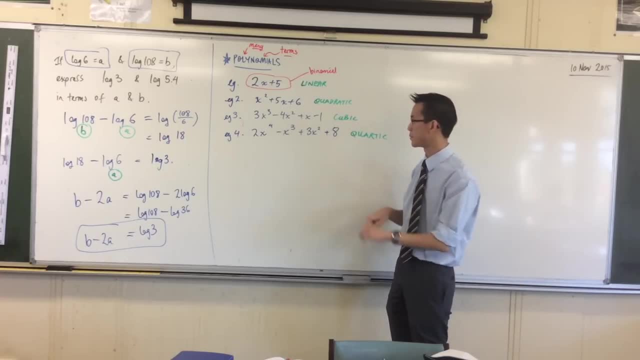 So 1,, 2,, 3,, 4.. These are particular kinds of polynomials. Now, to talk a little more specifically, there's all these different pieces in the polynomial that we know about. okay, One number is more important than all the rest. okay, 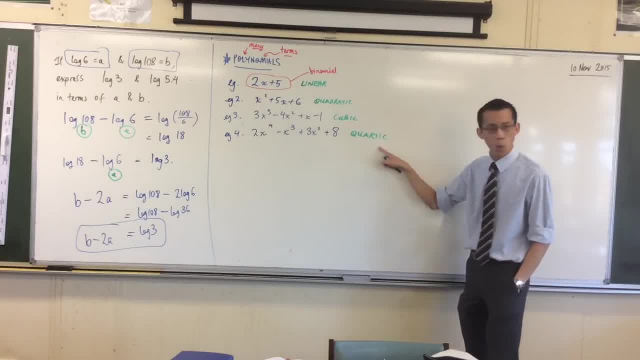 One number is more important than all the rest. I wonder if you noticed. See this quartic that I wrote down right. Do you see it's got a term here: x to the 4.. There's an x cubed. There's an x squared. 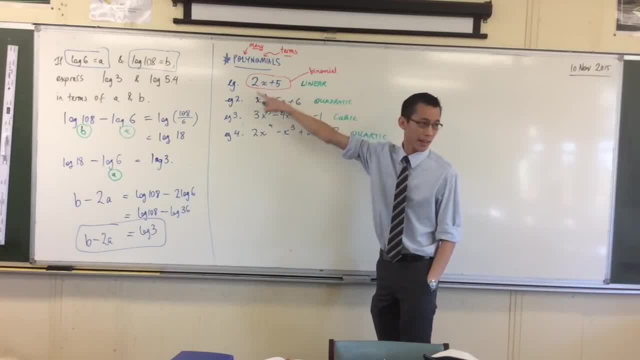 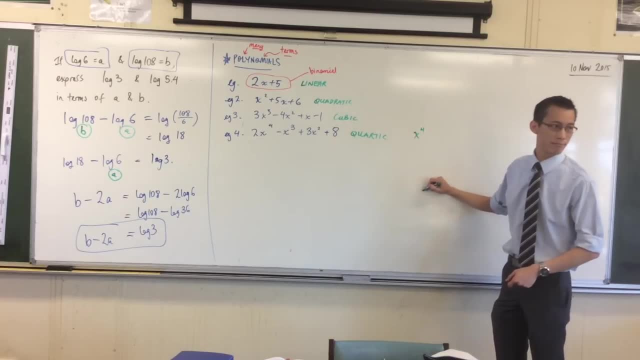 I don't have any x terms in there, Not like here and here and here. okay, But it doesn't matter, right? In fact, you don't have to write this one down. If all I had was that x to the 4,, it's already a quartic because it's got that number out the front there, right? 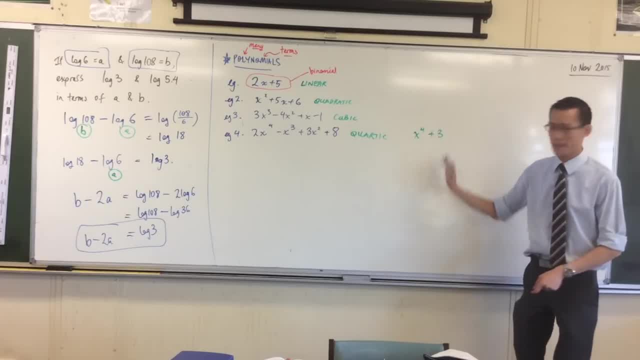 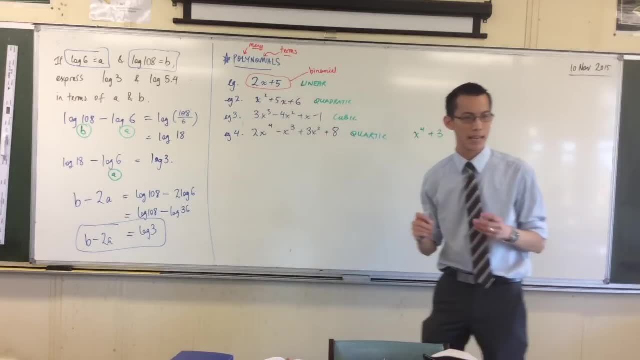 And you can add anything else to that that you like. These other things are much less important than that biggest number up there. whichever the biggest number is, It's kind of the one that takes the driver's seat and takes over and defines what's going on. 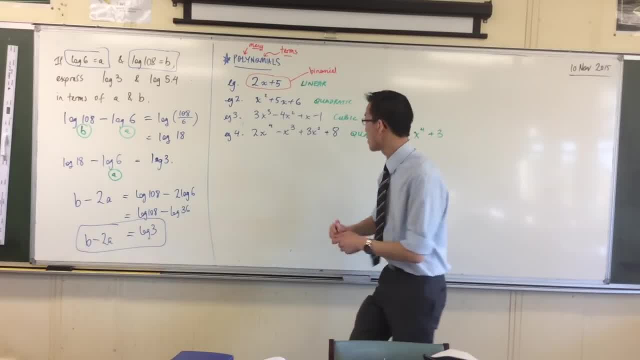 So therefore it's super important. We call that number. there It'll be 1 or 2 or 3 or 4.. We call that highest power, we call it the degree. okay, The degree is whatever is the highest power in your polynomial? 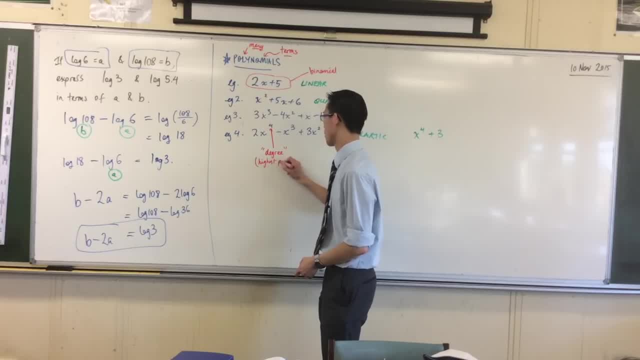 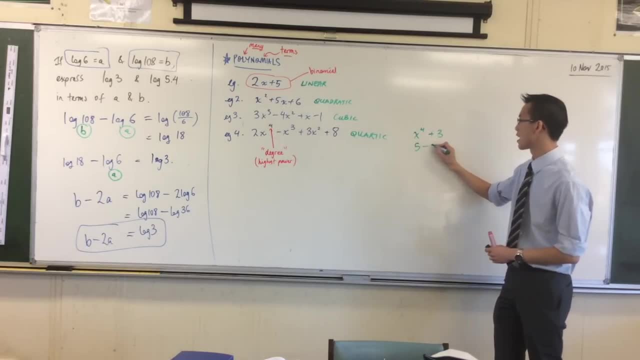 So I'll just write that That's the highest power you can find. It doesn't have to be out the front. You know I could write. see this guy here. I could write 5. take away x to the 4.. 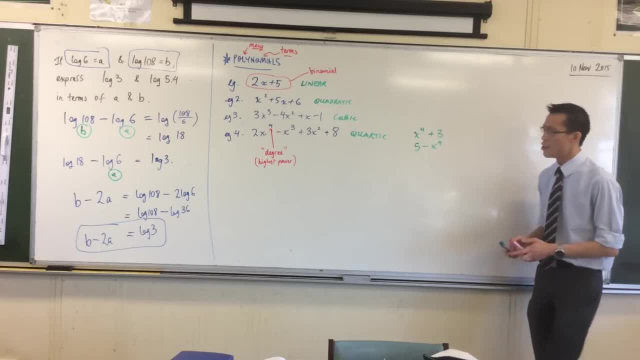 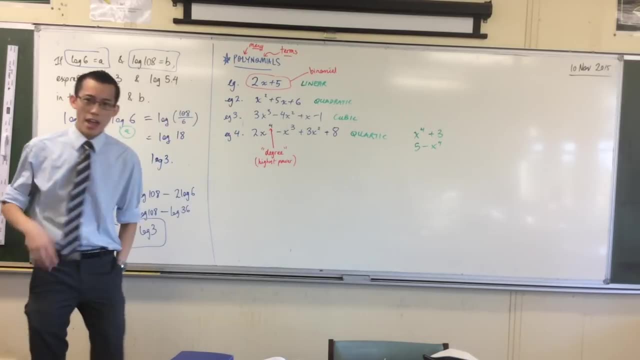 But the x to the 4 is the most important term. right, You can think about this in terms of functions, right? Remember, we said these are all functions. you can put a number in, you can number out. okay, If I put in numbers like, say, 0 or 1 or 2, really little numbers, okay. 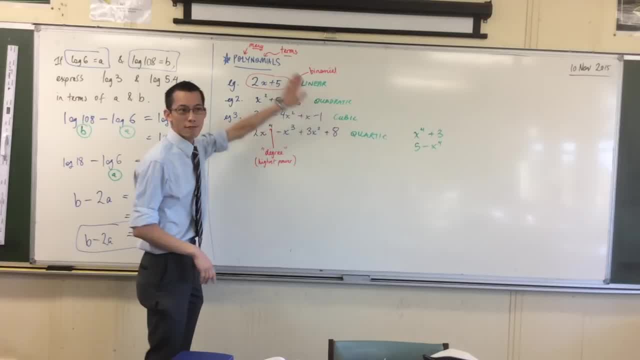 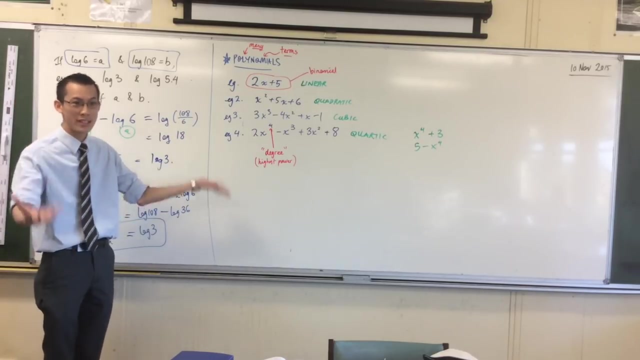 All of these numbers, on the end they really matter, right, Like 5 is a lot bigger than 0 or 1 or 2.. And 8 is a lot bigger than 0 or 1 or 2, okay, But if the numbers you're putting into your function are huge, if they're enormous like a million or a billion or a trillion, 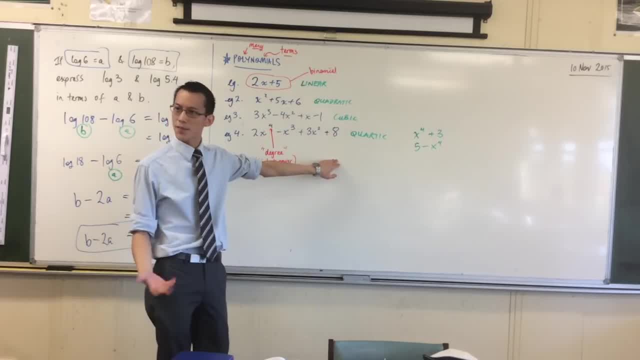 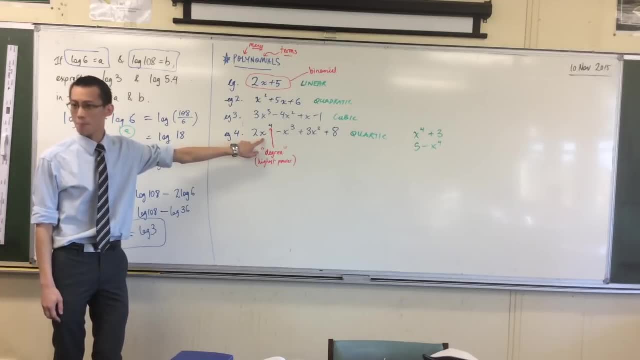 what difference does 5 or 6 or negative 1 or 8, what difference does that make when you raise it, you know, to the 4th power, And the answer is hardly any difference at all. okay, Like, if I'm looking at this guy, a million to the power of 4.. 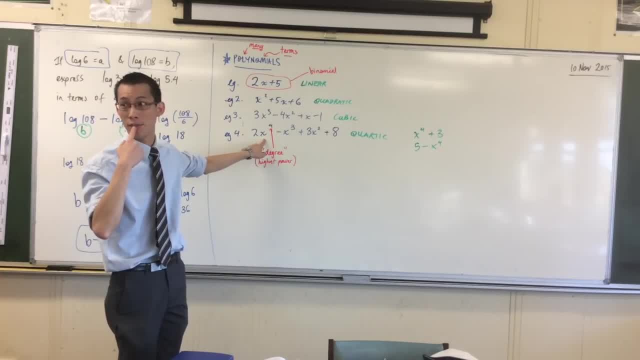 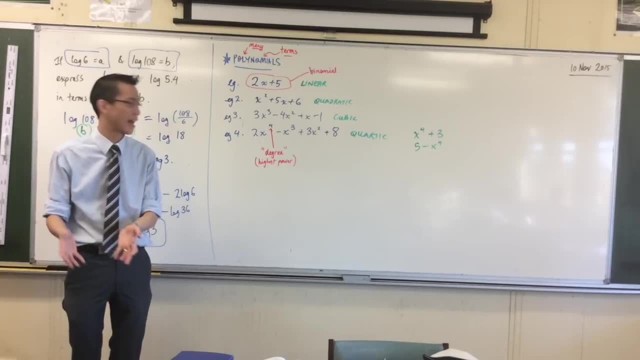 That's 1 with 24 zeros after it, And then there's an 8. We don't really care about the 8. He's so small, he's inconsequential. okay, Now, that's obvious. just with these numbers on the end. 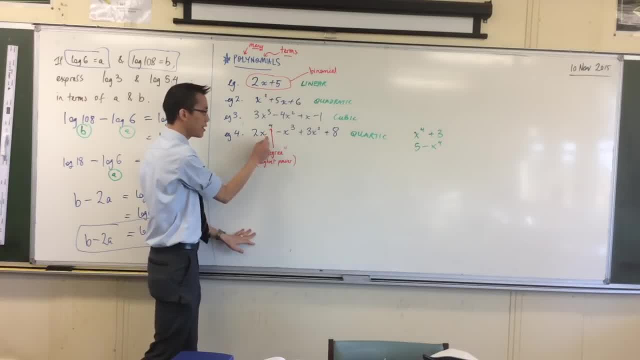 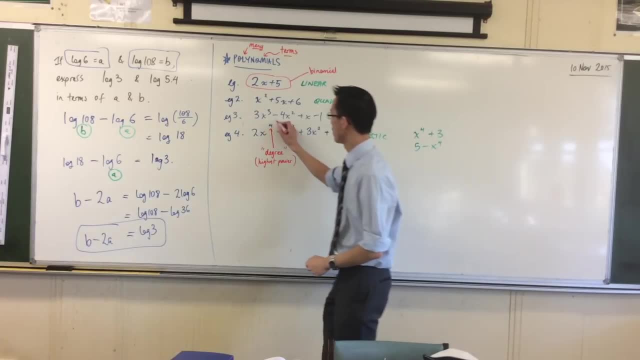 But in fact it's all of those terms. Only that guy is the one which really drives things, okay. So since he's so important, we attach a few other things to this right? So this whole term here. right, The one which has the degree on it. 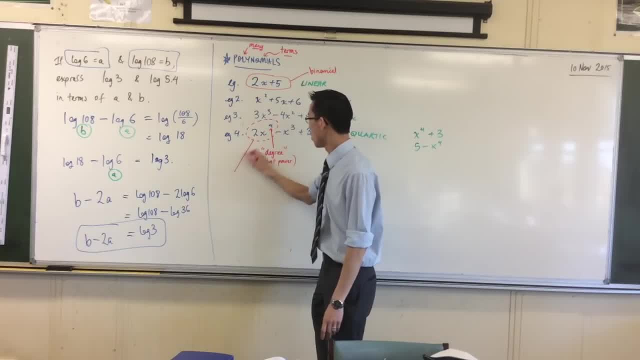 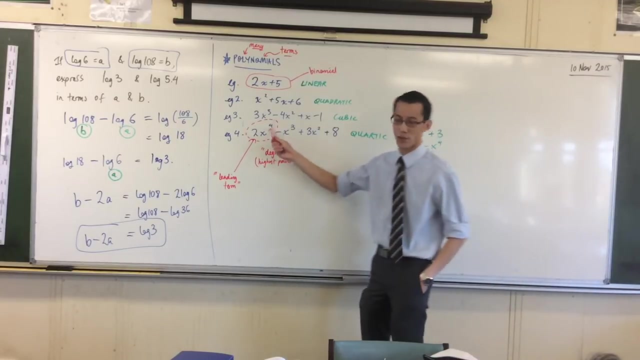 Remember I said a polynomial just means many terms. This whole term we call the leading term. It's the term that is the most important out of all the terms, right? I mean they all matter kind of okay, But this is the one which really makes a difference, okay. 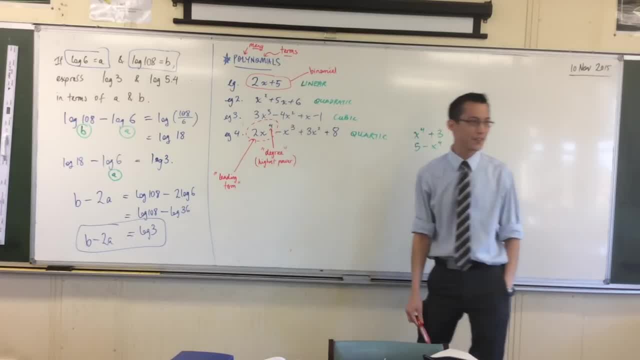 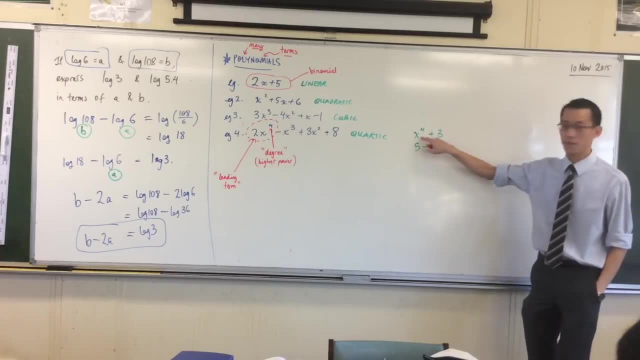 Because it's the leading term. the number out the front of the leading term is kind of important to me as well. For instance, see these two here: right, The leading term here is x to the 4.. The leading term here is minus x to the 4, okay. 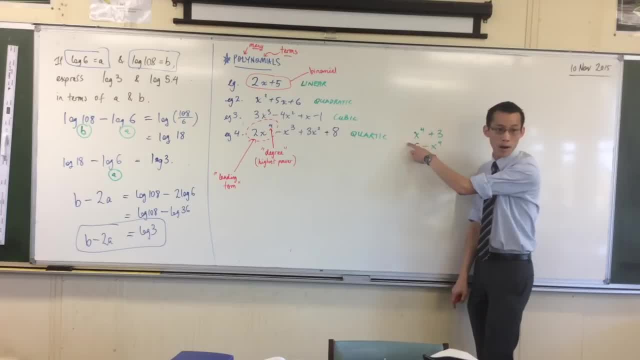 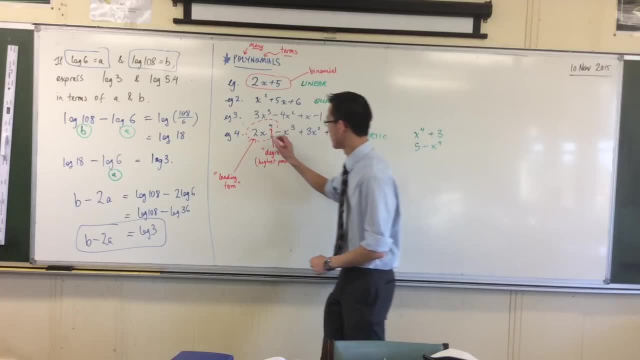 That number at the front, which in this case is minus 1, or in this case is 1,, makes a big difference. In fact, in this case it turns the whole thing upside down, okay, So, because that number is so important, I'm running out of space here, but I'm going to do it anyway. 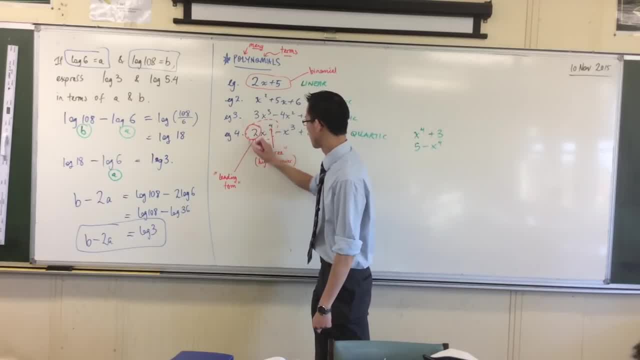 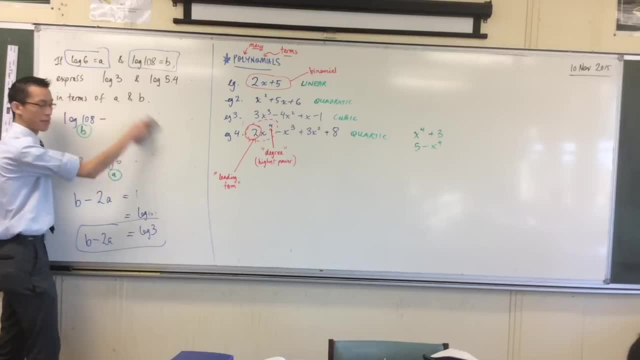 In this case it's a 2,. okay, I'm going to put it, I'm going to rub it out over here: The number in front of a pronumeral like x or y or theta or something like that is generally called a. does anyone know? Start to the c. 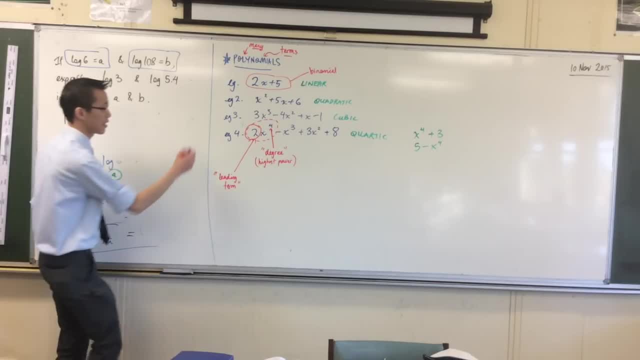 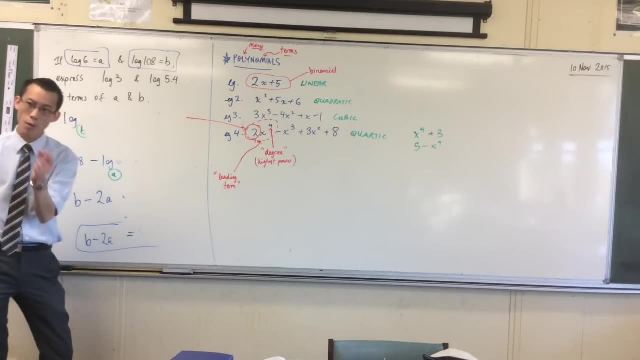 Coefficient. very good, We'll get to the constant in a second, okay, So this here. this arrow is going to the whole bubble, right, But just the 2, that coefficient- because it's on the leading term, we call it the leading coefficient. 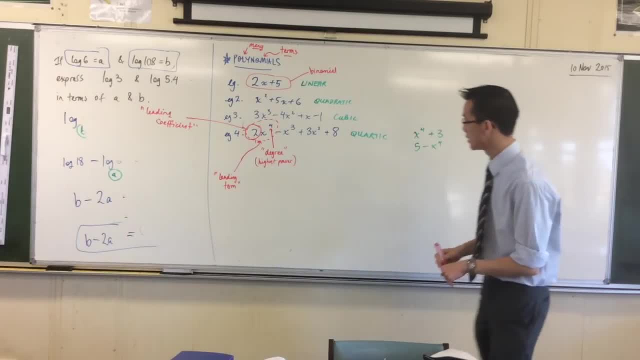 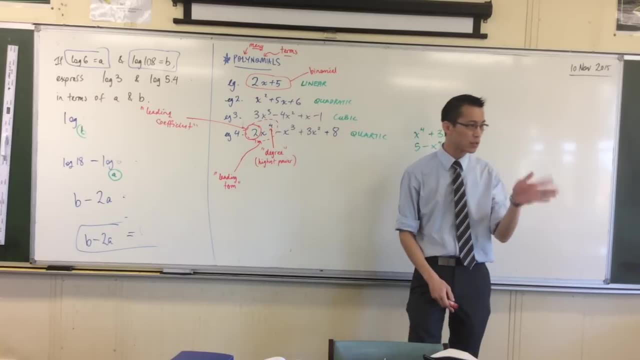 It's the coefficient on the leading term. Okay, Excuse me, You've got all these other terms. They have their own other coefficients. There's one more term that matters to me, which matters significantly enough that it gets its own name. 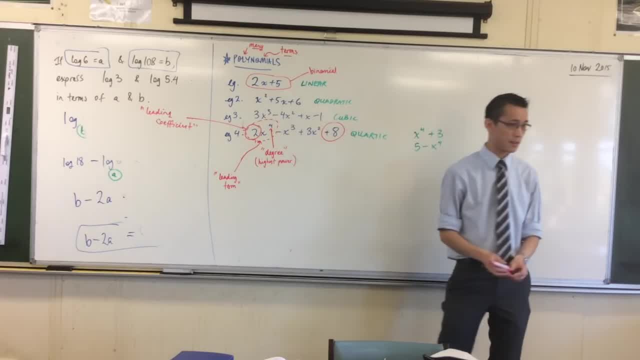 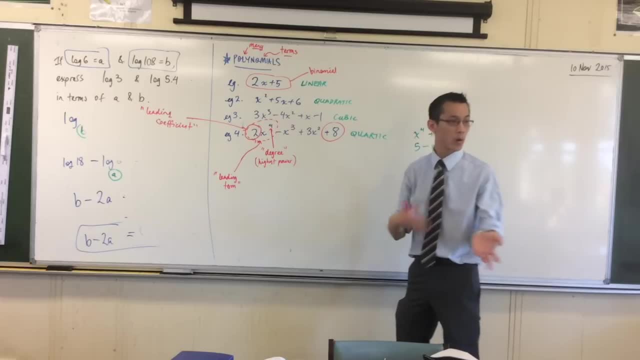 It's the one actually, this one on the end. Okay, this one on the end. Remember, a function changes its value depending on what inputs you lay into it, right, If it's 0 or 1 or 2 or 100.. 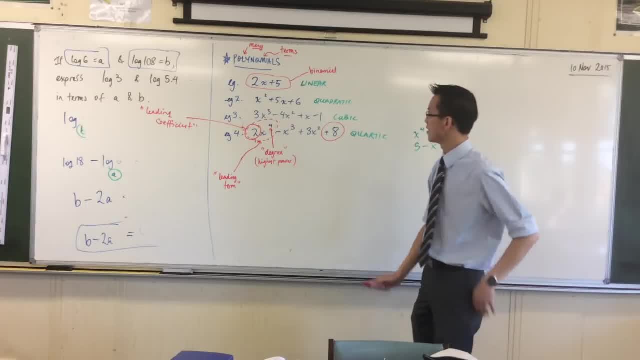 All of these bits with x's. they'll all change and they'll all vary, But this 8 and this negative 1 and this 6 and this 5, they don't care what x is Right, They don't get bigger. 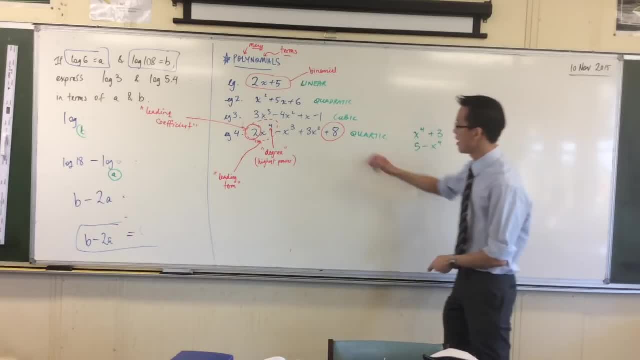 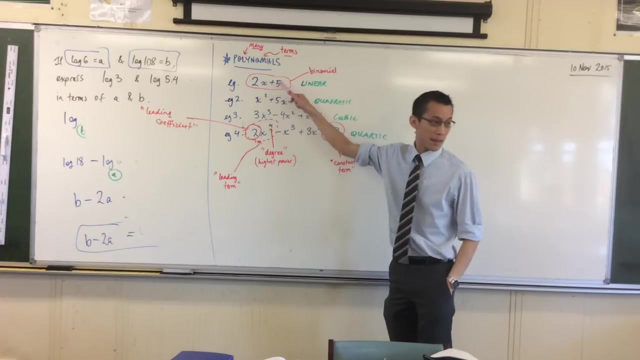 They don't get smaller. They're always the same size, no matter what x is. That means they're constant, They don't change. So in fact we call it the constant term. The constant term's really handy, right, Remember. in y equals mx plus b form like a straight line. the constant is just your. 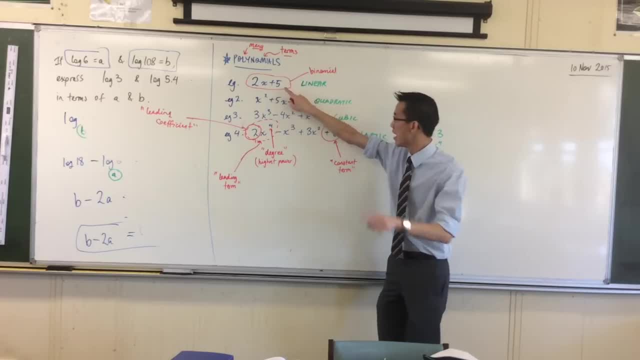 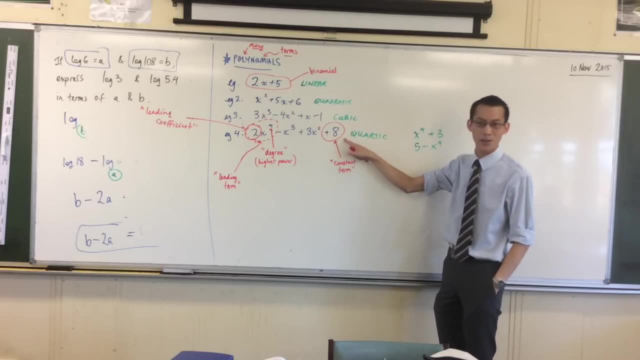 Your intercept, Y intercept. exactly right, In fact, the constant is always the y intercept. The y intercept of this quadratic will be 6.. And the y intercept of this cubic will be negative, 1.. And I have no idea what this quadratic looks like. 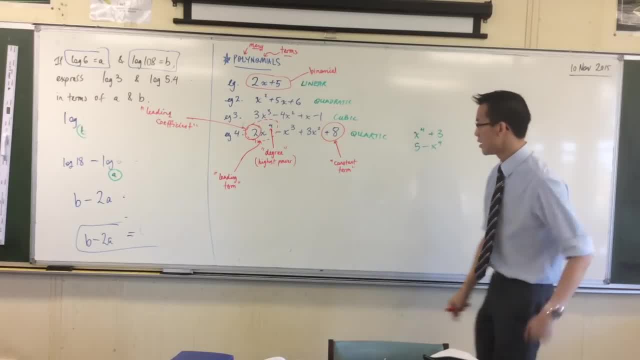 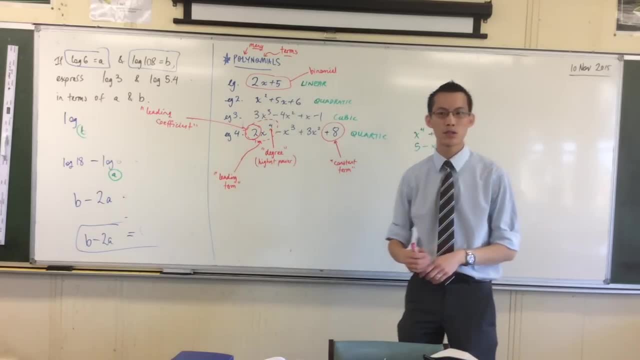 But I know its y intercept will be 8.. Okay, So here are our important pieces. These are like language that we're going to use and refer to over and over again as we do some actual operations on polynomials.